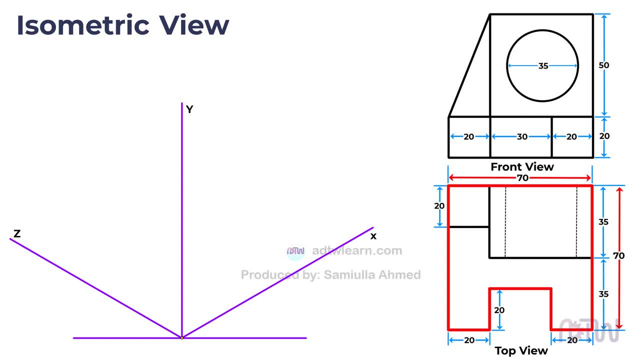 On the x-z plane. to ensure that the front view of the object is on the x-y plane, we'll position this corner point of the top view at this center point. Using a drafter, draw a 70 millimeters line parallel to the z-axis. 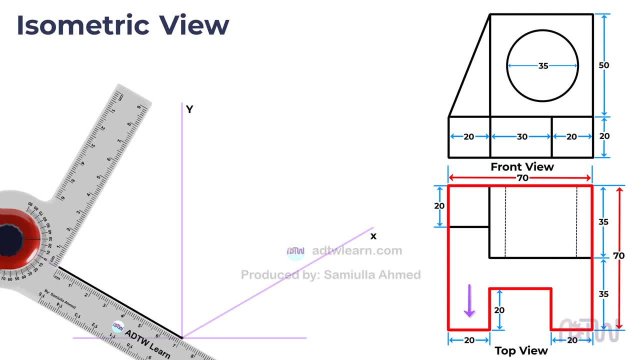 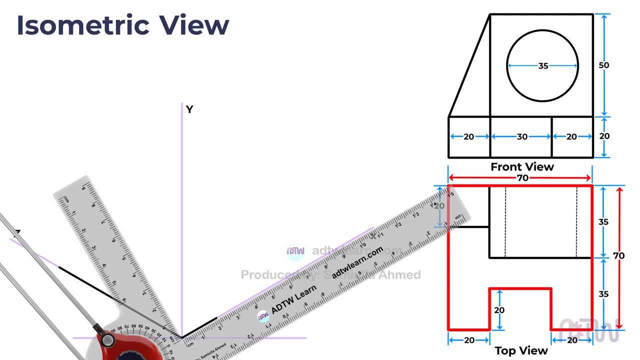 After this, we can see the width of this side is 20 millimeters. Take a drafter and draw a 20 millimeters line parallel to x-axis. Following that, we can observe that the depth of the slot is 20 millimeters. We can also draw a 20-millimeter line parallel to the x-axis. 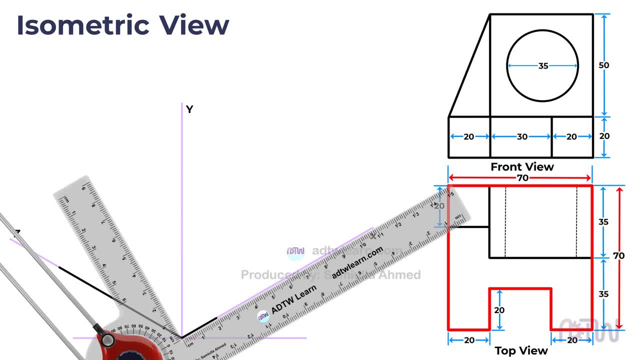 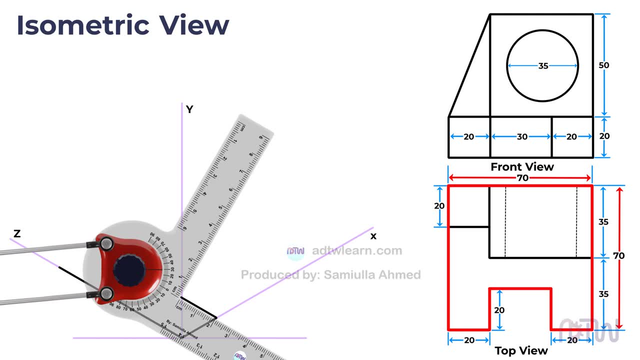 The width of the slot is also 20 millimeters. Therefore, we can draw a 20 millimeters line parallel to the z-axis. Additionally, the width of the slot is 30 millimeters. Thus draw a 30 millimeters line parallel to the x-axis from the end point of the previous line. 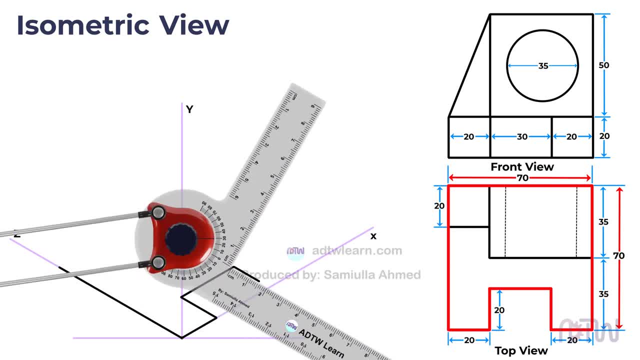 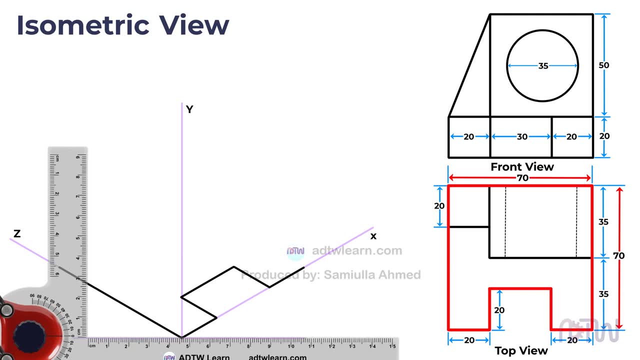 Next, draw another 20 millimeters line parallel to the z-axis, followed by a 20 millimeters line parallel to the x-axis. Then we notice that the total length of the object is 70 millimeters. Therefore, draw a 70 millimeters line from the end point of the previous line parallel to the z-axis. 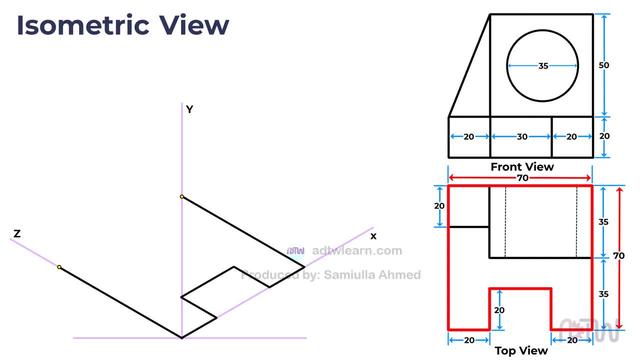 Finally connect the end points of both the lines to form the complete outline of the top view. This represents the outline of the top view Moving on to the next step. we notice that the thickness of the base in the front view is 20 millimeters. 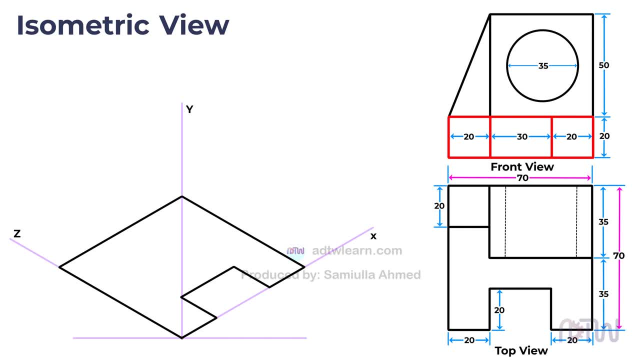 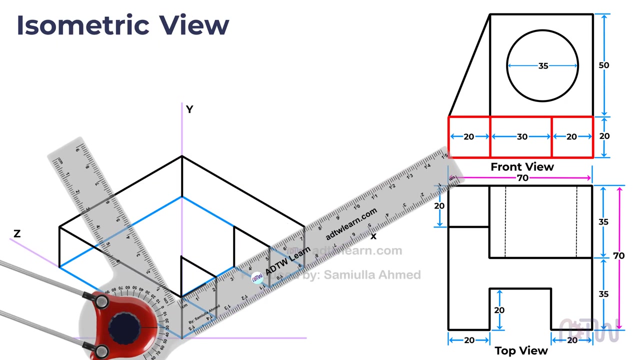 To incorporate this into our drawing. draw vertical lines of 20 millimeters from each corner point. Subsequently connect the end points of the vertical lines to form the base of the object object. Once we have established the base of the object, we can remove the additional lines that are. 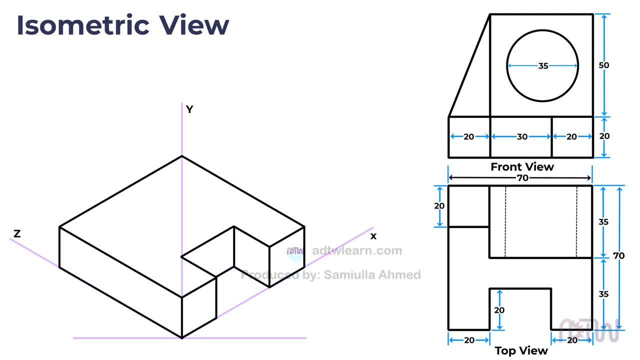 not visible in the isometric view. This results in the final isometric view of the object's base. Now we will draw the square shape on top of the base. In the top view we observe that the width of this shape is 35 mm and in the front view its length is 50 mm. Starting 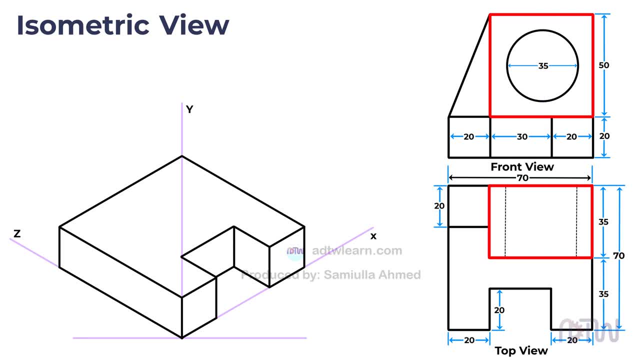 from this point on the isometric view, draw a 35 mm line parallel to the z-axis, Then draw another line of 50 mm parallel to the x-axis, connecting the endpoints to form a rectangle. Next, we note that the height of this rectangle is 50 mm in the front view To represent this: 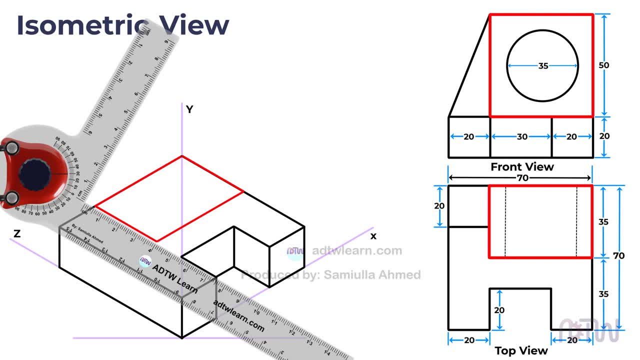 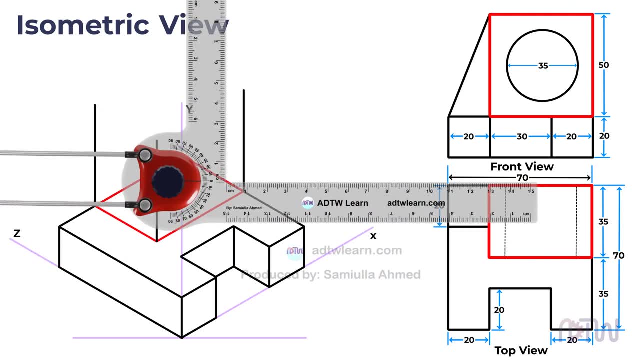 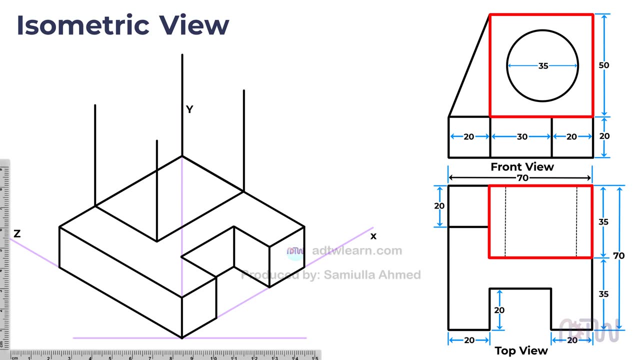 use a drafter to draw vertical lines of 50 mm from each corner point of the rectangle. Finally, connect the endpoints of these vertical lines to complete the square shape on top of the base in the top view. Moving on, we need to draw the inclined portion of the object. In the top view we can see: 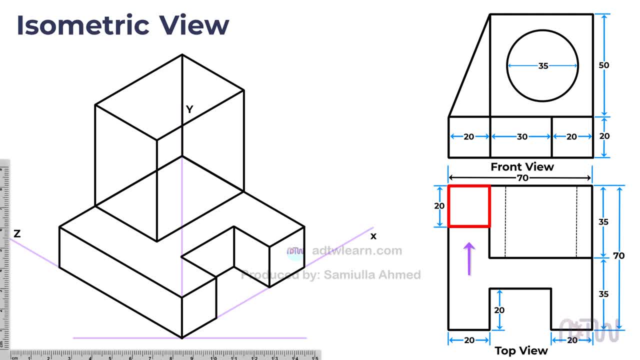 that the base of this portion is square. From the given isometric view, we can see that the width of this square is 20 mm. Therefore, mark a distance of 20 mm from this corner point along this line using a drafter and construct the square. 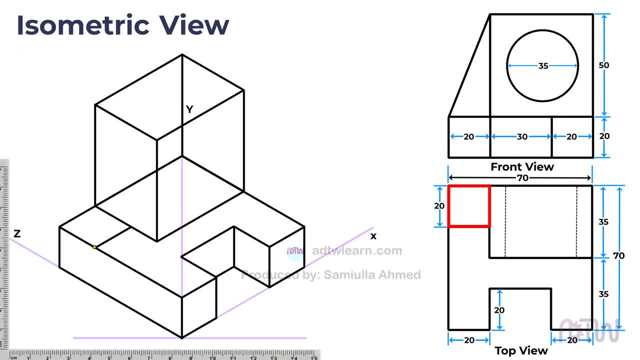 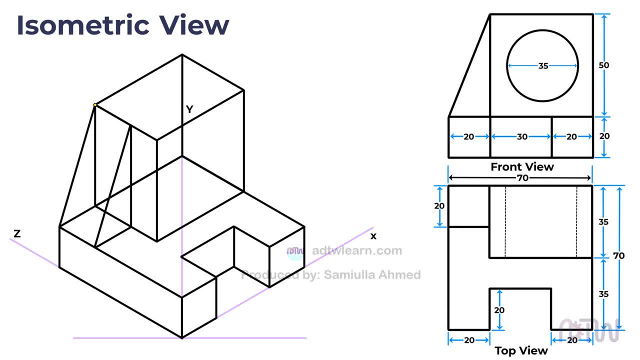 Then draw vertical lines from these points and parallel lines to the X axis. This will give us the required square with 35mm sides. Next, draw the diagonals on the square by joining opposite points of the corners. 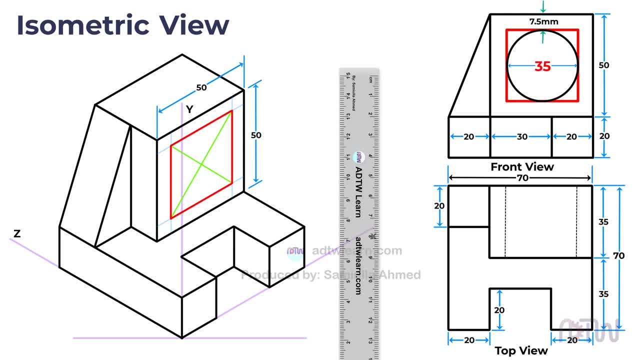 To find the length of the radius needed to draw the circle, we need to divide the side of the square in half. Since the sides of the square are 35mm, half of that is 17.5mm Mark points, 17.5mm away from each corner point of the sides. 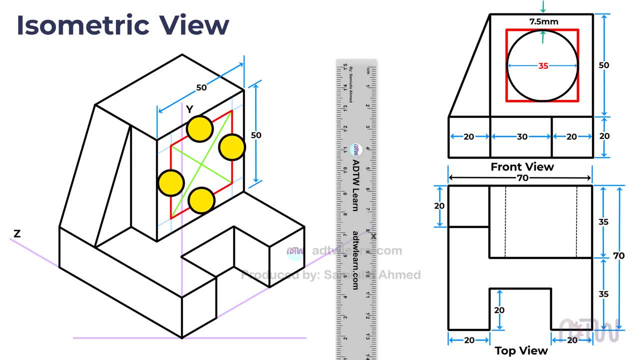 then join the endpoints of the smaller diagonal to the center points on the sides of the square. These center points will give us the length of the radius required to draw the circle. Take a compass using this point as a center, adjust it to this length and draw an arc as. 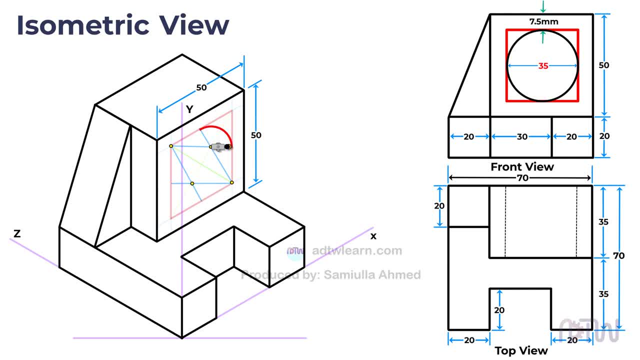 shown. Similarly, using this point as a center, draw an arc as shown Next. using this point as a center, adjust the compass to this length and draw an arc. In the end, using this point as a center, draw an arc. 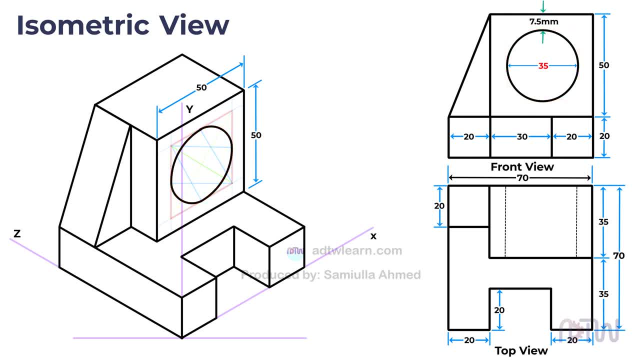 This is how the final circle looks in the isometric view. This is how the final figure looks in the isometric view. After this do the dimensioning of the figure. This is the final isometric view of the object. I hope this tutorial helped to understand how to construct the isometric view of an.